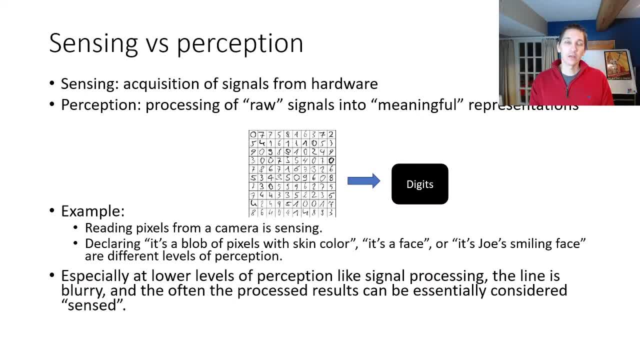 estimation process, step two. Now there's a bit of a subtle point here. I've used the words sensing and perception and at first glance they seem like somewhat like synonyms. Now in this class we're going to distinguish sensing versus perception as follows: Sensing is going to be the act of 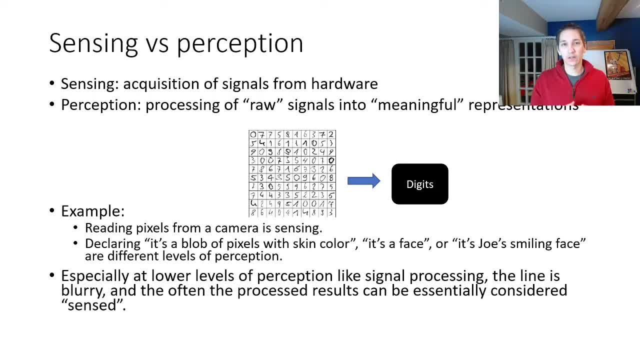 acquisition of signals from hardware, so essentially the way in which the signals are actually generated. Perception is the second step, which processes those raw signals into some sort of representations that are meaningful to downstream tasks. So, as an example, if we're trying to recognize digits from some sort of scan, the pixels themselves will be the sensing parts of 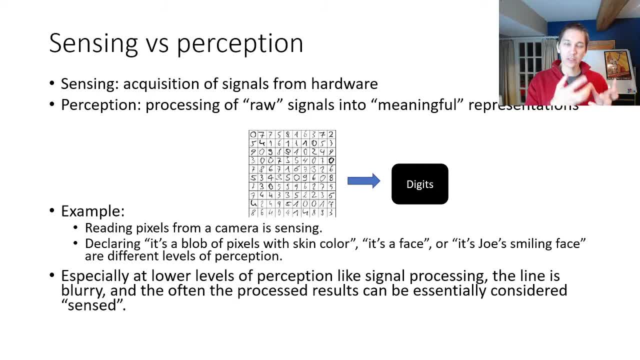 gathering the camera images but then detecting which digit that image represents is going to be the perception task. So there's different levels of perception in terms of different levels of sophistication of you know what is being produced for that downstream task. So, for example, if we're trying to detect humans, detecting a blob of pixels with skin, 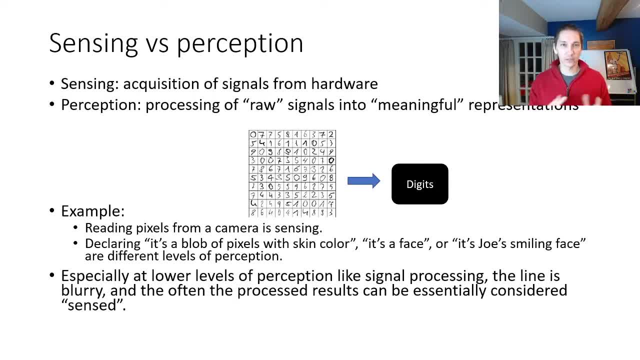 color is perhaps one form of perception which is fairly low level versus detecting a face, which is higher level, versus detecting whose face and what they're doing, which may be a much higher level input to some sort of planning algorithm, So near the lower levels of perception. 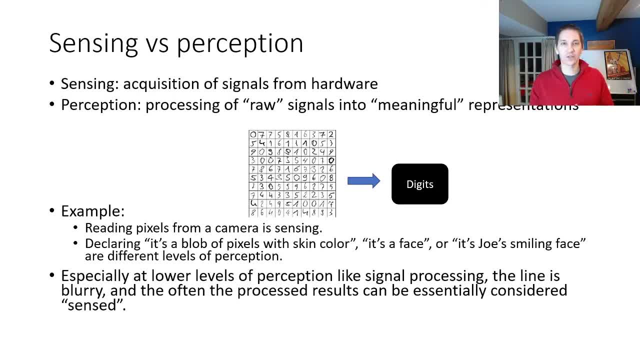 the line is somewhat blurred and so you can sort of, you know, discuss sensing tasks as essentially being low-level perception tasks, but in any case, you know, certainly at the higher levels of object recognition and so on, we're talking about perception. So the general way that we can think. 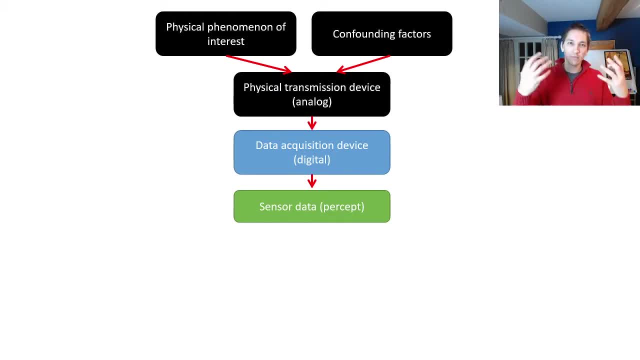 about sensing and perception is that the top few blocks here are involving sensing. So there's some sort of physical phenomenon of interest as well as potentially confounding factors driving the physics of some sort of acquisition device, the actual sensor. So there's going to be a physical 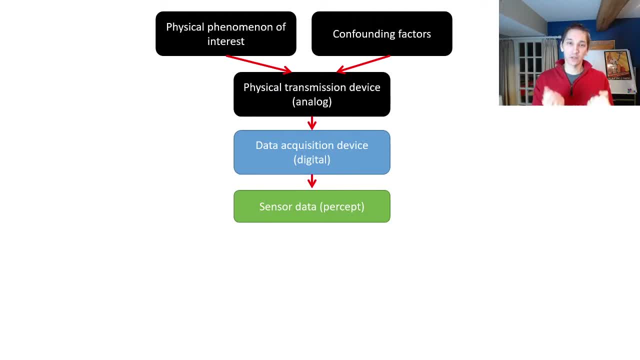 transmission to get those signals into some data acquisition device which is going to be digital, and then that is going to be then input into our decision-making system, our robot's mind, if you will. So this is all essentially part of the sensing pipeline. Then, after this data gets, 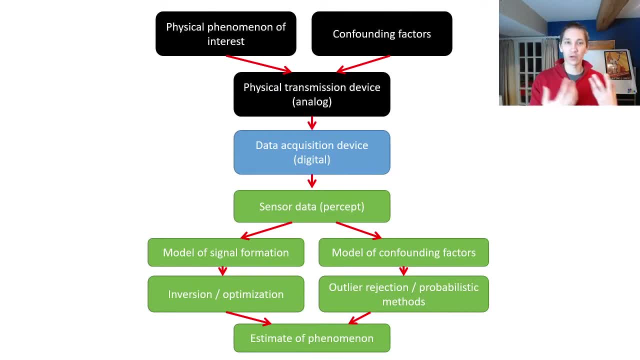 into our computer. we're going to be able to use some sort of model of this signal formation, a model of these confounding factors, and we're going to try to invert essentially the process that was given in the top half of the slide. So we're going to try to invert the process of this figure to try to estimate that underlying 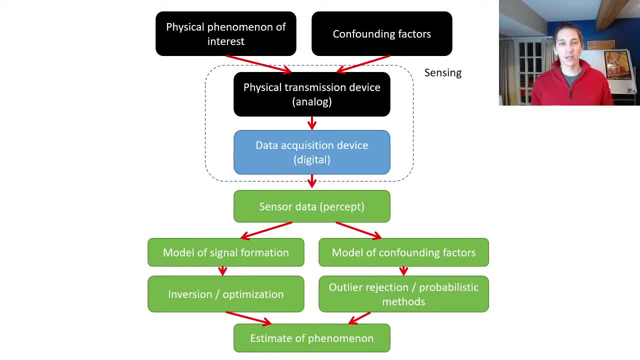 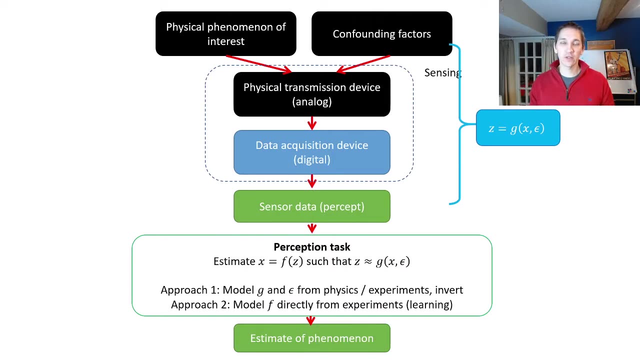 physical phenomenon. So, in any case, these blocks here are basically the sensing component, and then these blocks here are the perception component. So another way that you can think about this is that the first half of this diagram is some sort of forward transform which is producing our sensor data z from the underlying phenomenon of interest. 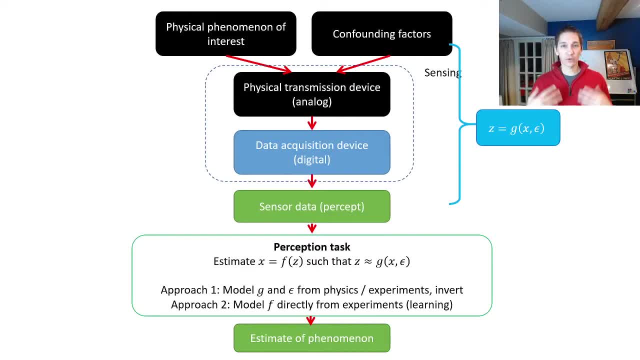 x, as well as some of these confounding factors. Epsilon, There's some forward transform g that we would like to then invert so that, given z, we can now estimate x. There's a couple of approaches for this. We could either try to model the g and 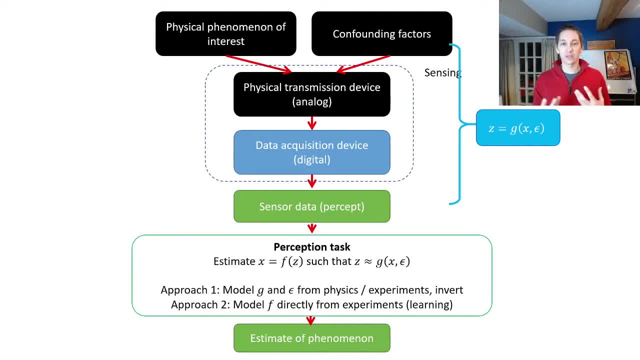 the epsilon from physics or experiments and then somehow invert this. So basically, using our own intuition and analysis, be able to construct this g function, and we'll look at some of these models that are used with this approach today: Epsilon. Another approach we'll be looking at much more in the future will be to try to model this function. 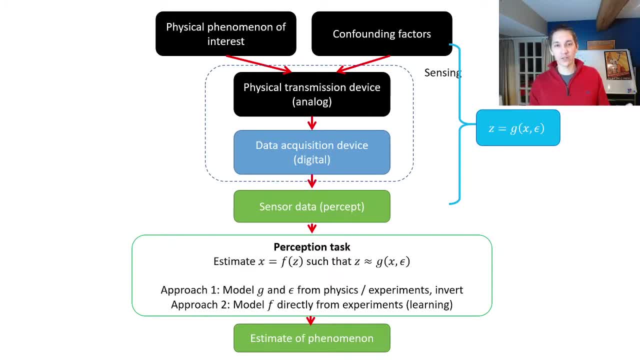 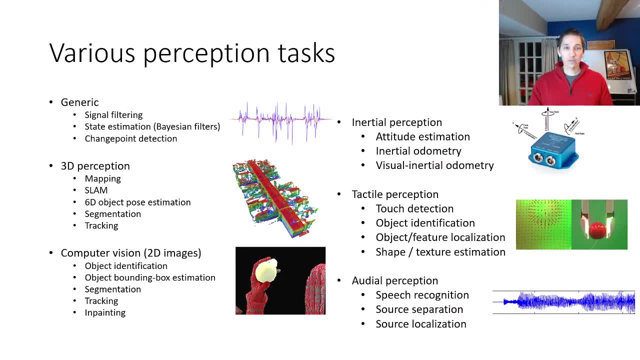 f directly through experiments. So if we have the ground truth x, we have the ground truth of z. try to just estimate f directly. Now there's also different types of perception tasks that fall into this framework. So in, for example, ECE classes, you'll be learning a lot about signal filtering, state estimation. 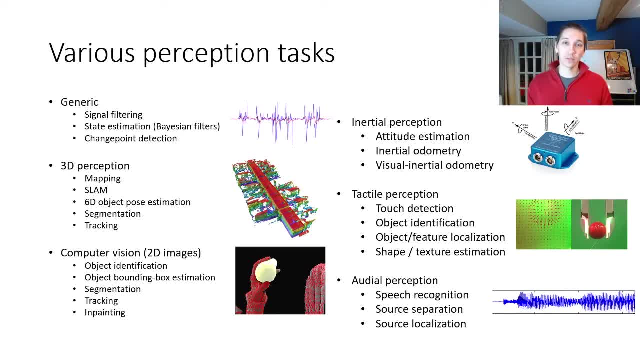 etc. We'll be looking a bit at 3D perception, in particular 6D object pose recognition and some segmentation as well. Now, with computer vision, we don't really think about 3D objects, but we think about images that represent 3D objects, And so, for example, object identification and 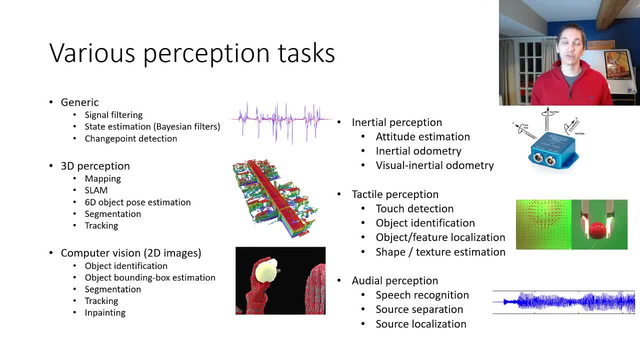 segmentation and tracking and so on are tasks that we'll look at with computer vision. In other robotics tasks you'll look at, for example, inertial perception or audio perception, which we won't look at in this course, but we'll talk about tactile perception using fourth torque. 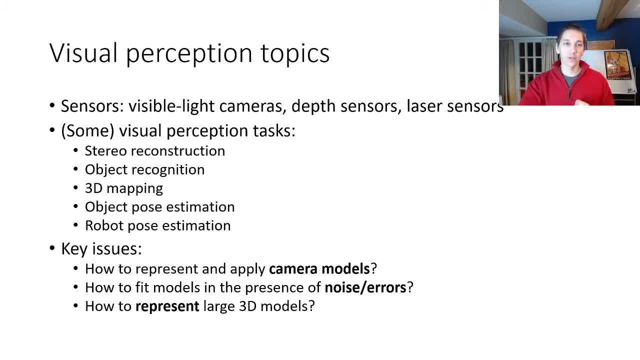 sensors in a later class start talking about visual perception. so these types of sensors, which are extremely rich and and also very low cost, include visible light cameras, depth sensors and laser sensors. we'll want to do things like perform stereo reconstruction of a 3d world. we might want to recognize objects. 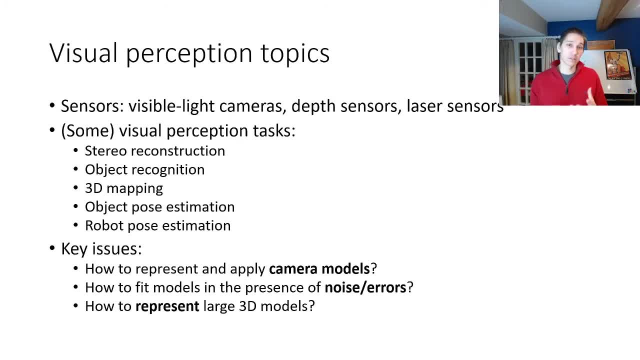 perform 3d mapping, also recognize objects that we've seen before and where they exist in our scene, and we may also want to understand how our robot is interacting with those objects. so the key issues that we'll talk about today, and also subsequent lectures, include: how do you, how do? 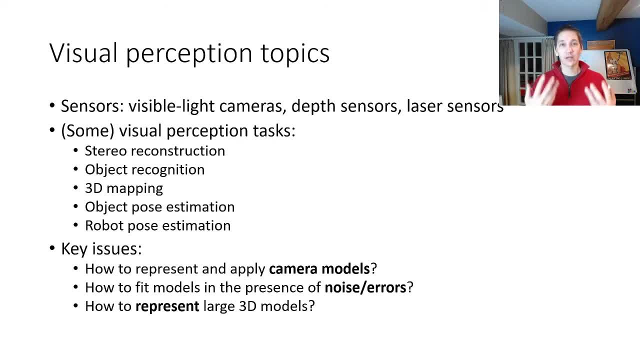 we model cameras and how do we then apply these models to estimate quantities of interest? how do we then fit the models in the presence of noise and errors, which will be the topic of next class and calibration, and we're also going to talk about representation of of 3d models as well. 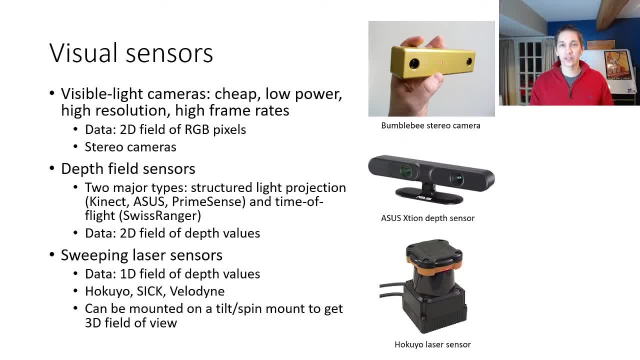 so various types of sensors that are quite inexpensive and available- uh, you know- essentially off the shelf, include visible light cameras, which will give you an image, of course, at usually 60 frames, 30 frames per second or 60 frames per second, and there's also stereo cameras, which give you a pair. 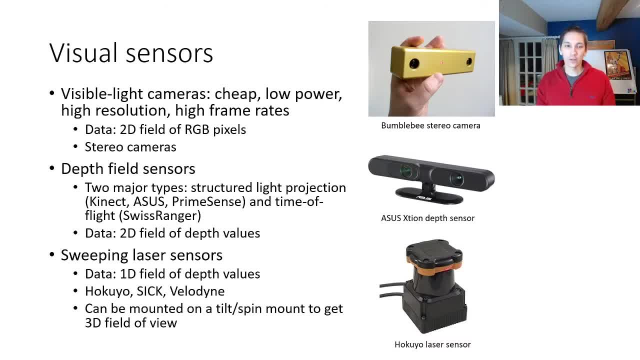 of these visible light images. there's also depth field sensors which try to give you a an image of depth, basically distance to the camera, but slightly different than distance it's. we'll talk about that subtlety in just a few slides, but in any case there's two major types of such 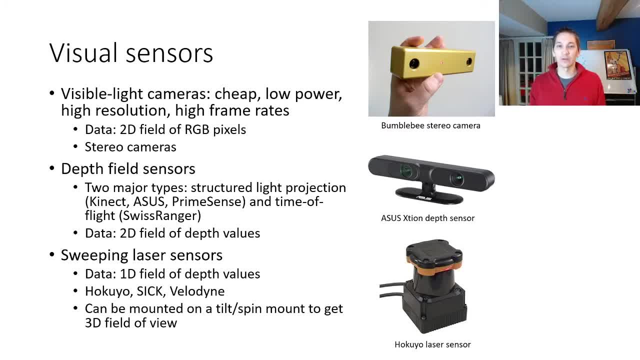 cameras. there's structured light projection as well as time of flight, which use lasers to determine the distance to the camera. there's also laser sensors that sweep a laser across a scene, and these laser sensors use time of flight to figure out the distance to the to the sensor, and typically these are one-dimensional signals. they basically sweep in a. 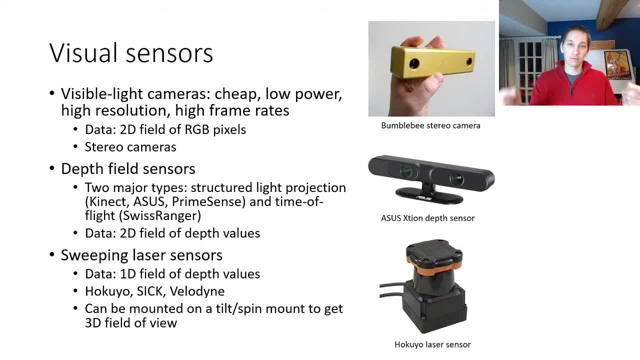 certain angle and give you this kind of one-dimensional value set of values of distances, uh. now, if we want to get three-dimensional uh values, we can mount them on a tilt system or a spinning system and that will allow us to get three-dimensional perception of points in our roulette's environment. so sensors vary in their 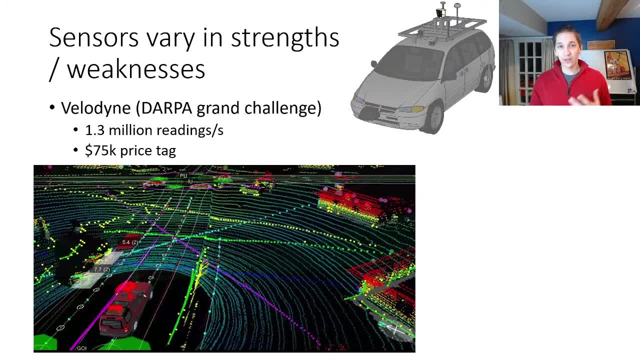 strengths and weaknesses and there's no perfect sensor. back in the good old days of the darpa grand challenge, which precipitated a lot of the current work in autonomous vehicles, some of the top teams were using these velodyne laser sensors that spun around and gave you multiple channels of 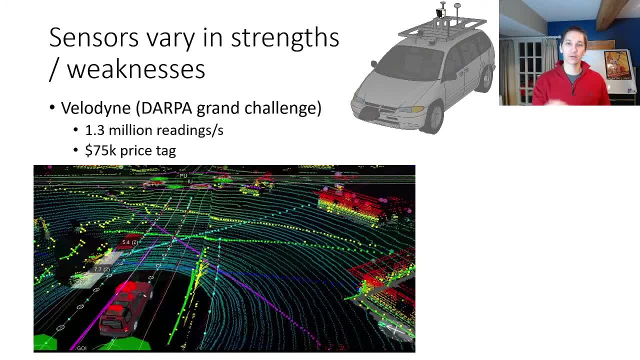 readings in the vertical and horizontal direction of the sensor, and they were able to get three-dimensional access, but then provided 360 degree view and also very long maximum distance readings. these gave 1.3 million readings per second, and they also came with the downside of a very hefty 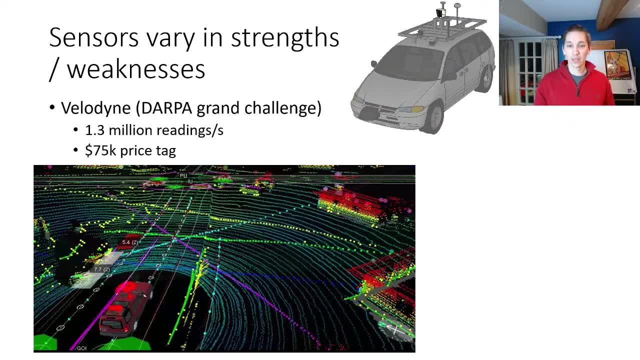 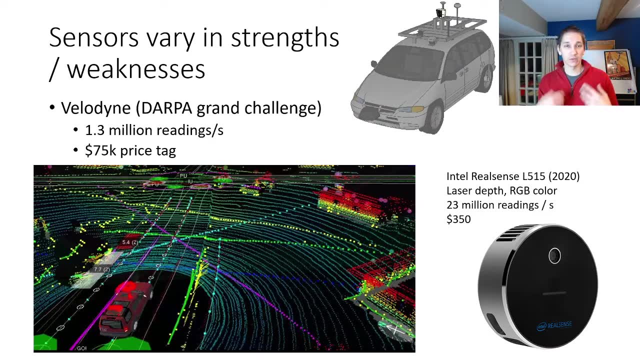 price tag of 75 000 each. now, fast forward to today. we can buy, for example, the intel realsense l515. this uses lasers to provide a depth image at 30 frames per second, as well as rdb color, and you can get 2.3- sorry, 23- million readings per second at the cost of 350 dollars. now, uh, this has some. 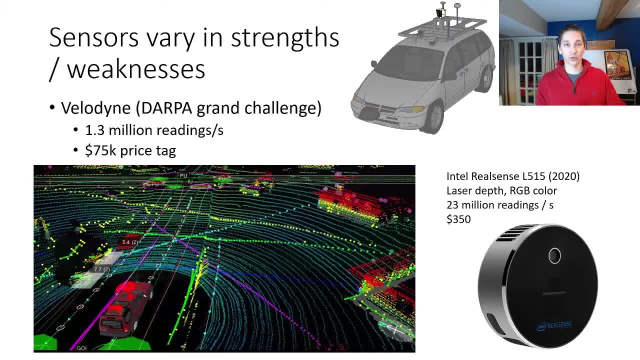 disadvantages in terms of its maximum range being much shorter- i think it's approximately eight meters- but in terms of manipulation, this gives us very rich depth readings and very- uh, dense reconstructions of 3d worlds that are kind of in a kind of robot manipulation scale. 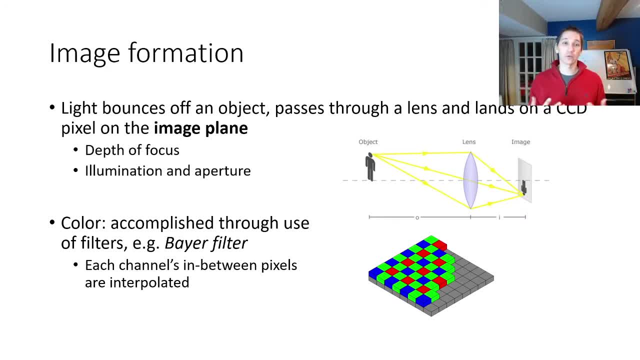 okay, so let's think about how to deal with images and work with images. basically, we'll be looking at basic camera modeling. so, in general, to get light into a camera, light bounces off some object. it goes through the lens of the camera and then lands on some ccd pixel. this pixel will be on some plane called the image plane. there are various. 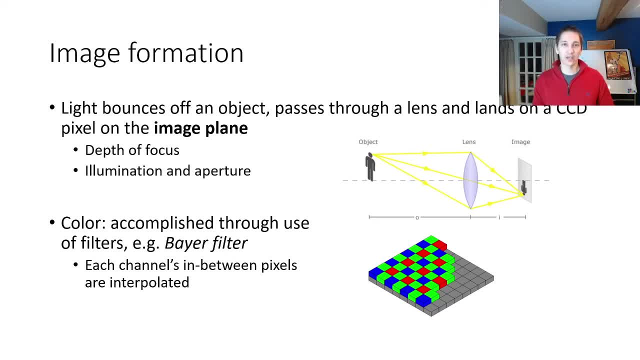 issues regarding lensing that need to be taken into account, such as the depth of focus, illumination, but for many cameras, these are essentially automatically adjusted for whatever type of application is being uh being addressed. if you're into photography, you'll look more, much more deeply into these. uh, the lensing topics. uh, for the most part, in robotics, we tend to have 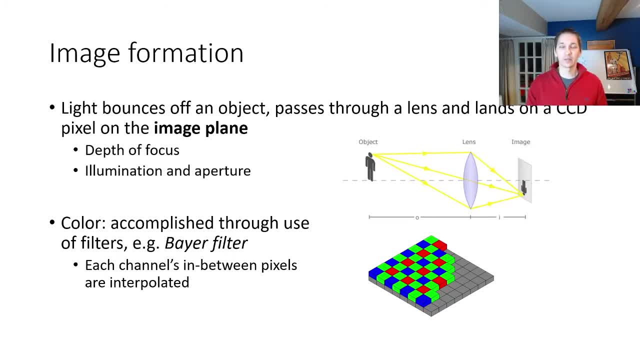 very small cameras with very small lenses, and these tend not to be so much of an issue. one thing that may be interesting to you is that cameras don't directly sense colors. they actually just sense light intensity, and in order to get color out of your imaging sensor, we use filters such as the bayer filter. 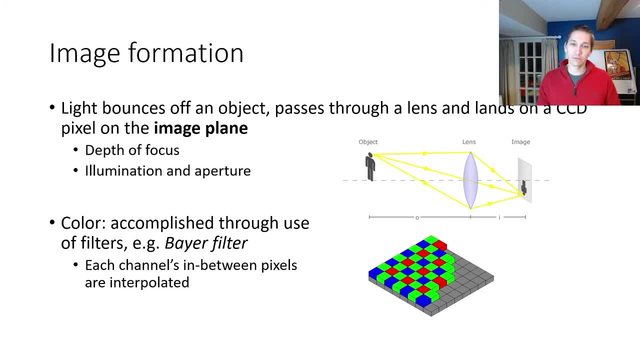 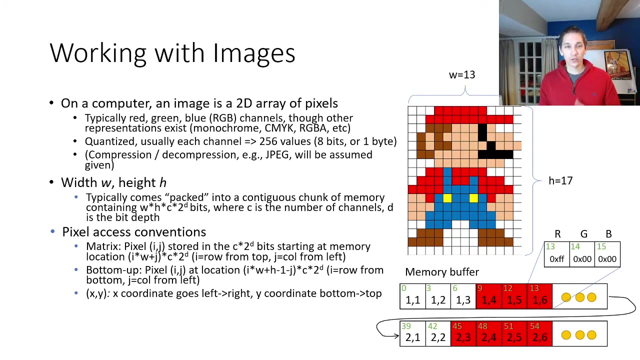 which takes basically a grid of red, green and blue filters to only let certain wavelengths of light through. now, with the intermediate pixels, we're going to interpolate the full red, green and blue colors by by doing some sort of interpolation between neighboring pixels. so in order to work with image, we have to understand how to deal with addressing of. 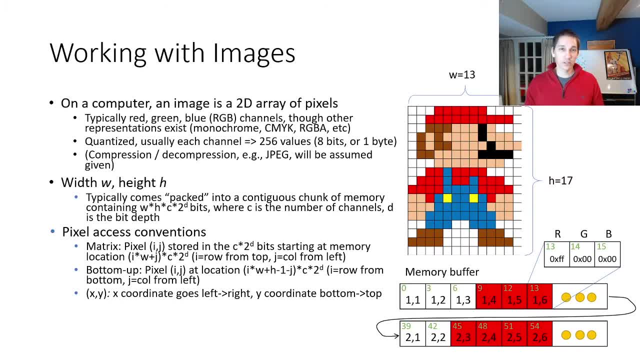 these, these pixel arrays. we want to think about images as two-dimensional arrays of colored squares, these pixels. we typically work with red, green and blue representation, although if you're working with, for example, printing, you may also be using, like cmyk, colors, etc. these are going to be the light. intensities are going to be quantized typically to 256 possible. 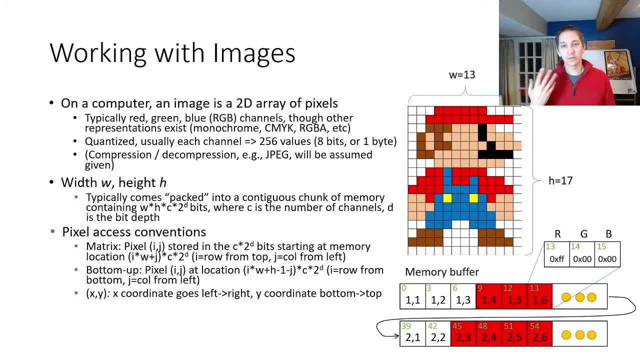 which is also one byte, and oftentimes, well, we we want to work with what's known as uncompressed images, which is basically a full matrix of images, and many times you have jpegs, png type of file formats which actually compress the images. typically, when you load, then you'll decompress. 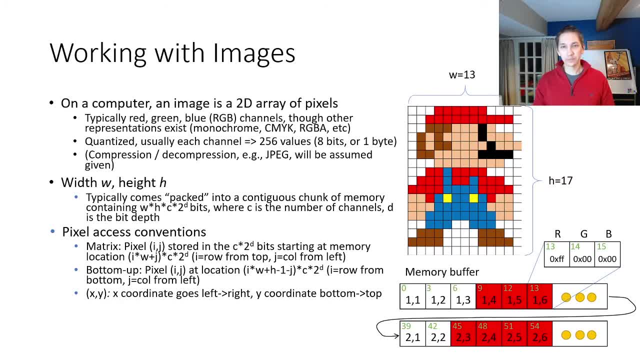 them into this kind of array based format. the array will have some sort of width and height, but these will typically be packed into a contiguous memory buffer containing h, d, 2, p, c, and d happens to be 10 to the px. so now, if we're trying to access a given pixel, you have to be aware of the type of pixel access. 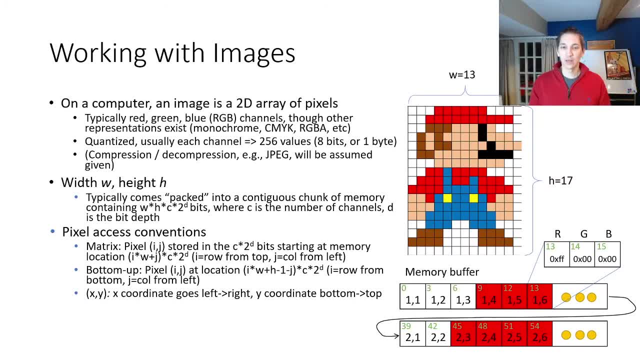 times w plus j times the size of the pixel. So this is where the pixel starts. The pixel itself will include some number of channels. So, for example, this red block over here- 1,, 6, is going to be red, And so it's going to have three bytes. The first byte is going to be 0xFF. 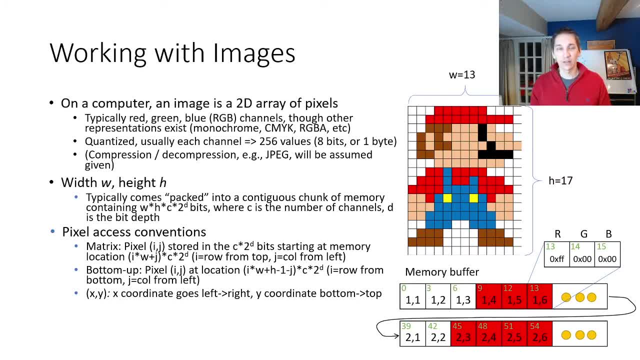 which is the maximum value there, 255.. And then the green and the blue are both going to be 0.. And you should also note that sometimes there's different pixel access conventions. So, for example, certain conventions use bottom-up representation where the row actually goes from. 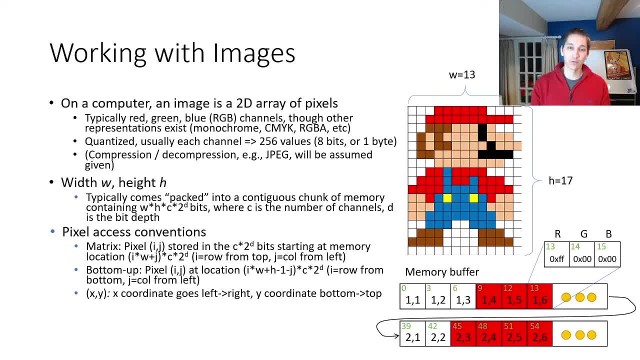 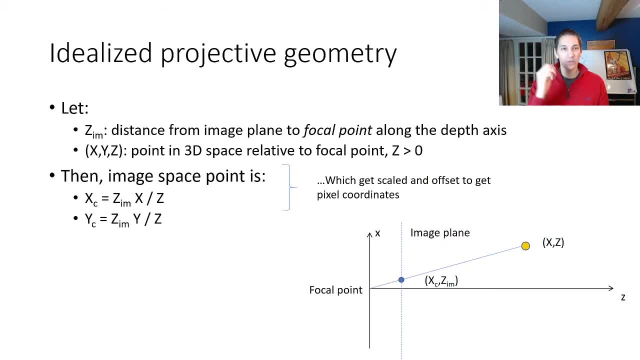 the bottom to the top, And there's also xy convention, where the first entry goes left to right and the bottom entry goes bottom to top. Now, how does this correspond to stuff in the 3D world? Well, so we need to model how cameras form images, And we typically do so. 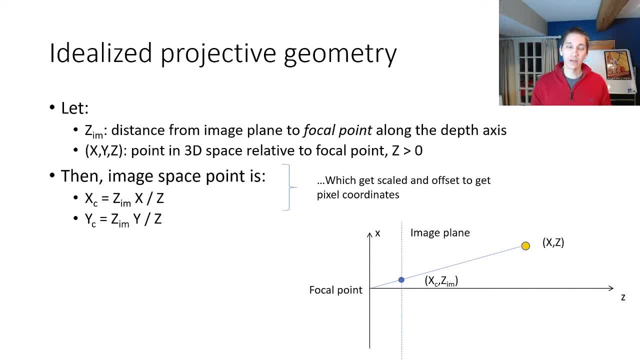 using what's known as idealized projective geometry. If we have an imaging sensor on an imaging plane some distance away from the focal point of the lens, then we can model the transformation of the light coming from that point through the lens to the image sensor as a projection transform, So through the rule of similar triangles. 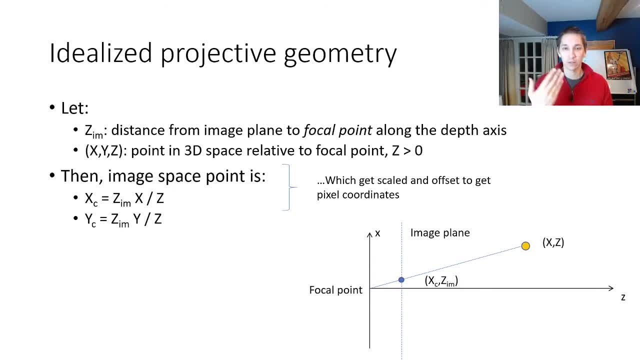 the image space point xc here, which is basically given as a sort of coordinate on the image plane in terms of real units. But on the image plane it's going to be the distance from the image plane to the focal point, times the x coordinate divided by z. So that's going to give you one coordinate and there's a. 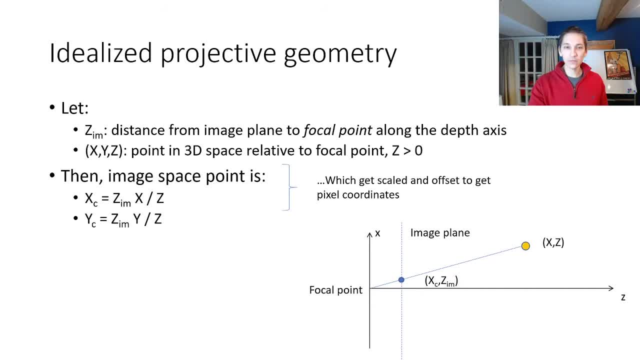 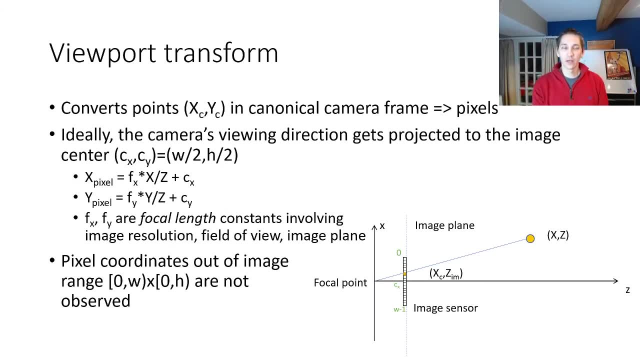 simpler transform in the y dimension. Now, in order to get pixel coordinates, we're going to scale and offset these using the next transform here, which is known as a viewport transform. So, given those real points on the image sensor, we're going to then see which one. 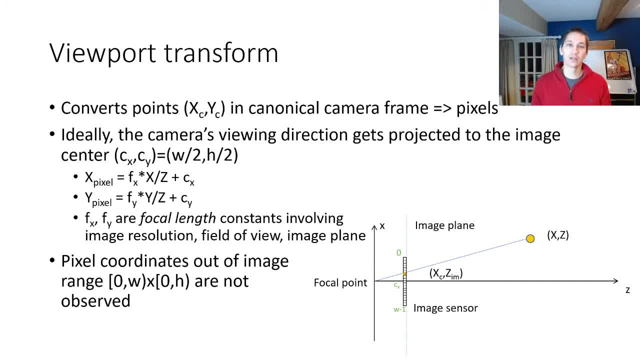 which one of the pixels on the image sensor actually gets activated by that light ray. So the point xc, yc gets converted to a pixel by a scaling and an offset. So there's an image center which corresponds to the 00,, you know direct forward direction of our camera, And there's also 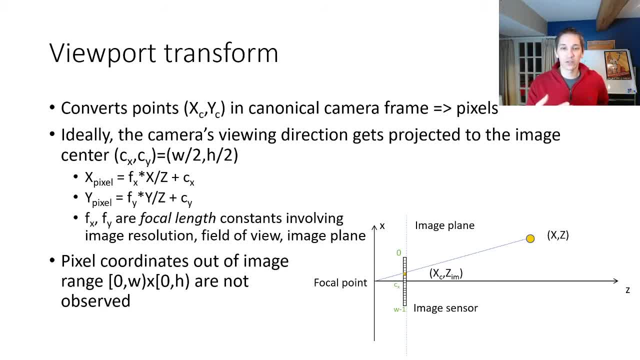 going to be a scaling that has to do with the image size as well as the field of view and the length of the image plane. So essentially, the overall transform that gives you the pixel coordinates is going to be some f times x over z plus some offset cx. Now, if you had a point that went outside of the image range, 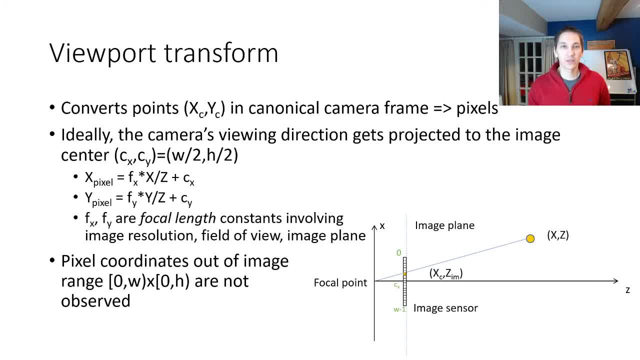 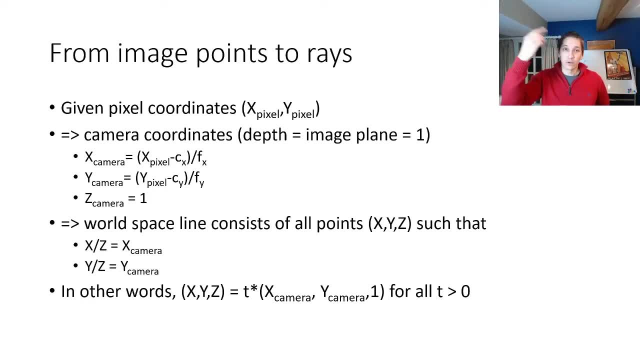 then it's basically not observed. So you also want to sort of clip things to the inside of this viewpoint. Okay, so we oftentimes want to do the reverse of image formation. we want to figure out what in the world generated this pixel that we see. So if we have a pixel coordinate x, y, then we can. 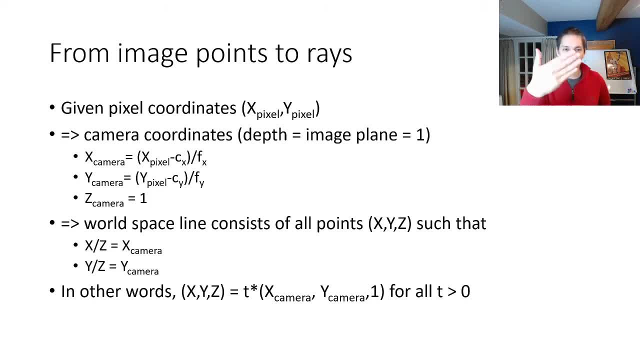 convert to the camera coordinates, if we assume that the image plane was at one unit away from our focal point, And then we can figure out the world space line through that, that point, which means that given the x pixel, y pixel, we can convert it to the x, y, z of that target point and then any 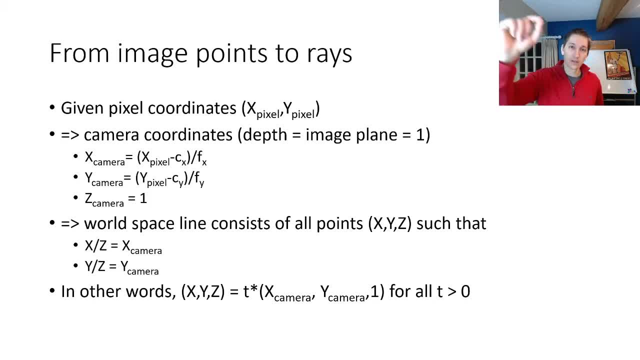 point along that ray between the focal point and that computed point- x camera, y camera, z camera- any point along that ray is going to potentially be the generator of that pixel. So there's a bit of redundancy here, you know. if you know, if I see something at a certain distance, something in exactly that ray. but 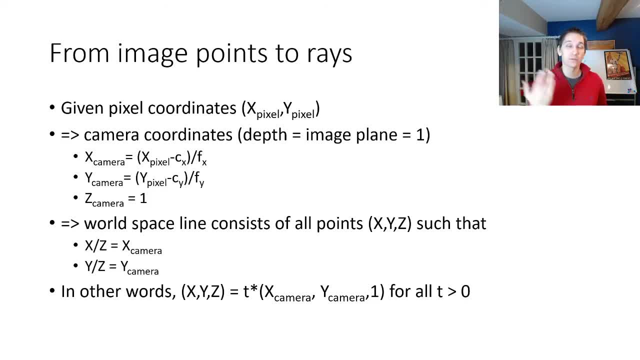 twice the distance with the same intense light intensity will generate the same light intensity on my eye, And so this is a subject of a lot of you know possible, for example, optical illusions that you know play with your sense of scale and and depth. 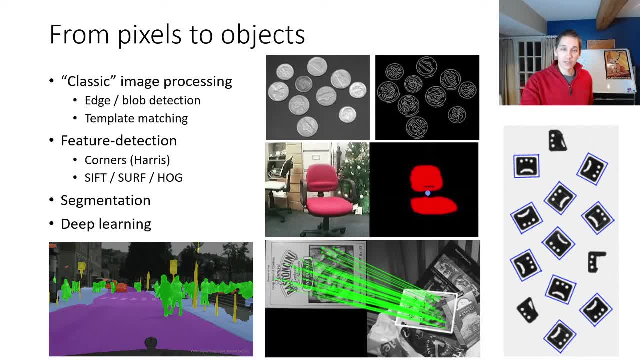 estimation. Now we oftentimes not just want to, we don't just want to go from pixels to points in the space, but we also want to recognize objects in the scene, And we'll talk about this when we get into computer vision. So there's lots of different types of computer vision algorithms, ranging from 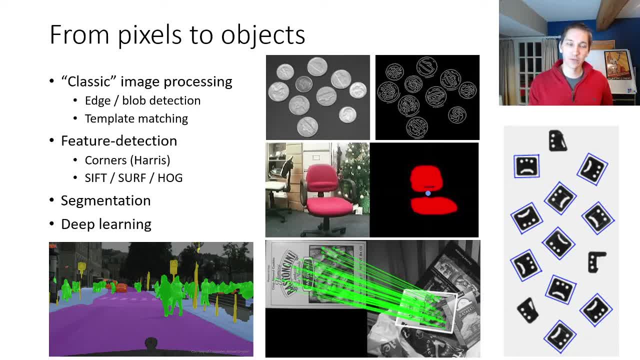 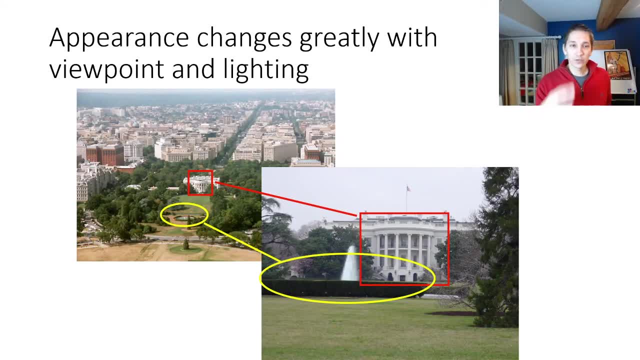 classical image processing to feature detection algorithms, segmentation algorithms as well as deep learning approaches, And so we'll get into this in a future lecture. The really tricky part about computer vision is that appearance really changes greatly depending on the viewpoint and the lighting conditions. So, for example, this slightly 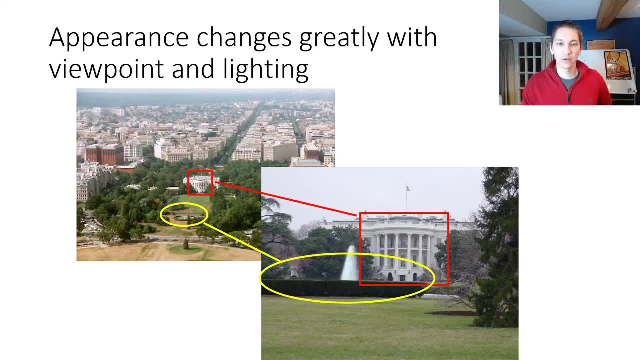 overhead view of the White House that's taken from fairly far away is very different from the image that we see on the right here. So you can see that in the first image it takes up a tiny part of the image. there's also a 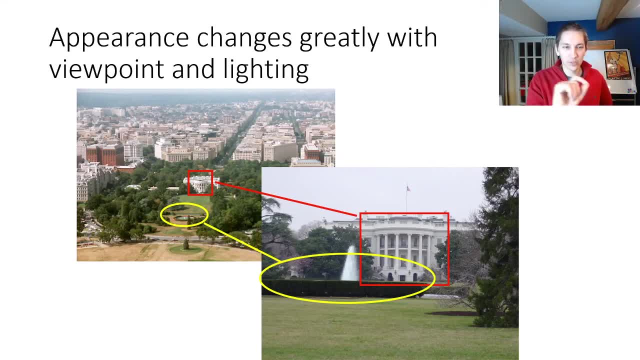 distance, a fairly large distance between the pool and the front And the building itself. But if we see a image taken from the ground, this square is taking up a much larger part of the image. the pool is taking up a huge part of the foreground. it's even sort of blocked and doesn't even. you can't even see the water from here, But you. 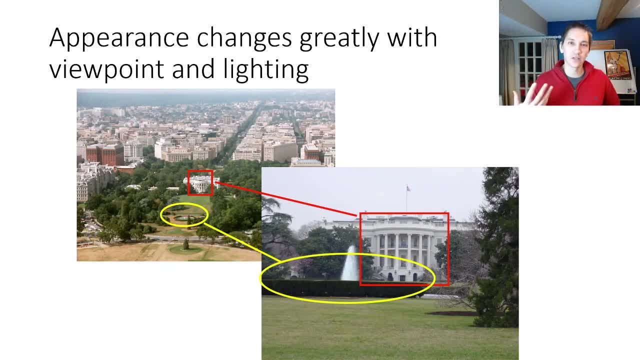 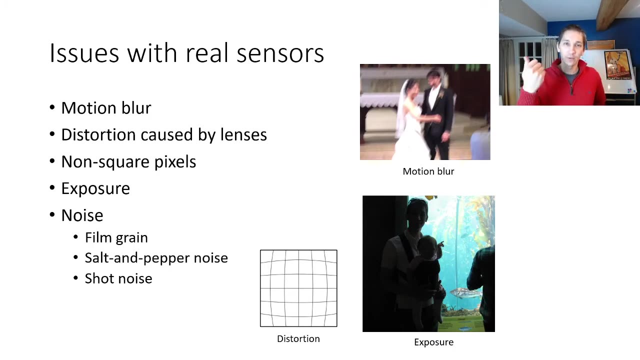 know. if you want to, for example, be really reliable at recognizing an object, you have to be able to develop algorithms that will be tolerant to these changes of the viewpoint, as well as lighting conditions. There's other image issues that we have to deal with with real sensors, especially when we're dealing with images taken from robots. 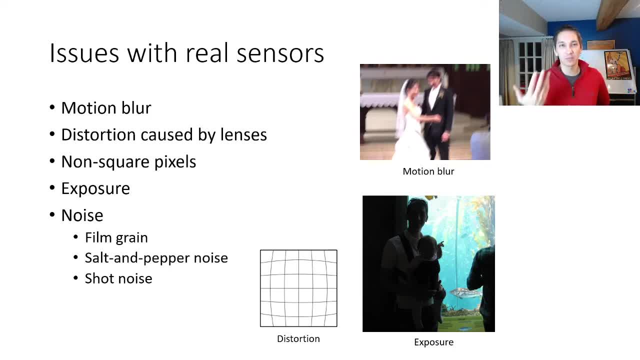 because oftentimes, when we're talking about computer vision, you're oftentimes taking pictures that people have selected based off of photographic intuition, So we'll oftentimes toss out images that have poor exposure or motion blur etc. But we can't control this so well on our 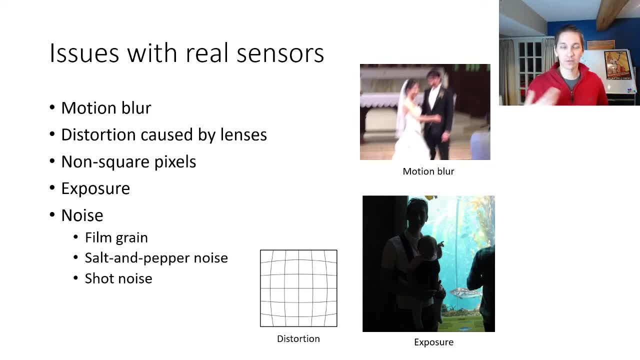 robots, And so here we have to worry about these types of things and develop algorithms somewhat specifically for robots if we're going to make them reliable, especially for, for example, moving robots or robots that need to work with very different lighting. 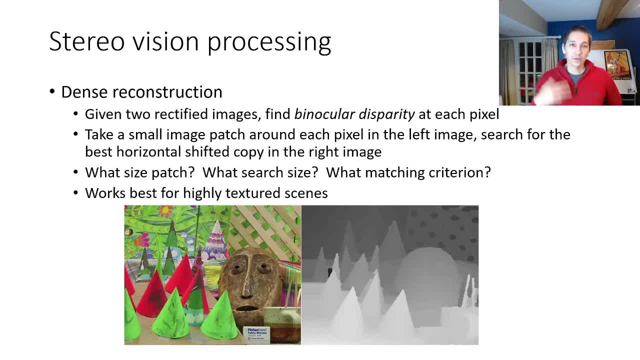 conditions, A couple of other tasks that are used. So, for example, stereo vision processing is trying to construct a three dimensional representation of the world, given two sensors. So if we take two images that are slightly offset from one another, these are called the offset. 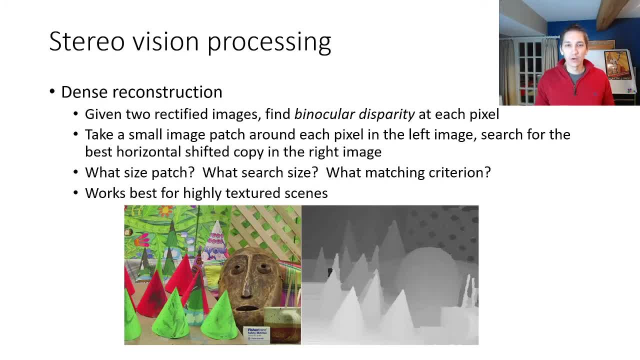 between them is called the baseline of the stereo pair. If we see the same object from each of these these, these cameras, there's going to be an apparent offset in the horizontal direction. that will give that's known as the binocular disparity. So you can test this out by putting your finger in front of your eye, closing one eye and then switching to the other one. you can see. 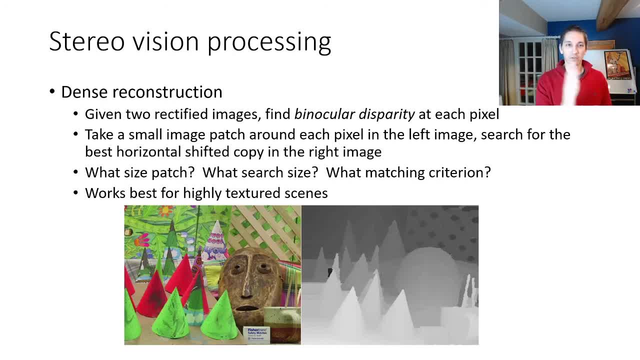 your finger switching in apparent position from left to right and vice versa. So the idea is that we can- if we can recognize some part of the image on one image- usually two images, taking the left image into account as the reference- and then find the same patch in the right image, then we can try to search for how much that has been shifted. 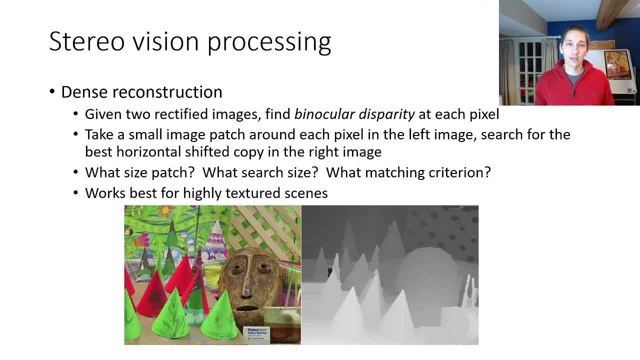 And then this corresponds to the depth by an inverse transform. So the less binocular disparity you get, the farther the object is away. Now there's a lot of different complexities in terms of building dense reconstructions, in terms of the algorithms for performing matching, etc. 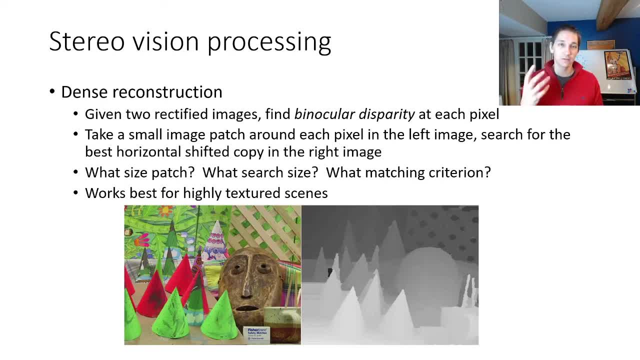 But there's a couple of aspects of stereo vision that are very common. One is that they perform much better in textured scenes than untextured scenes. So if you looked at a wall, for example, that was completely blank, stereo vision would do very poorly because it can't find good matches. 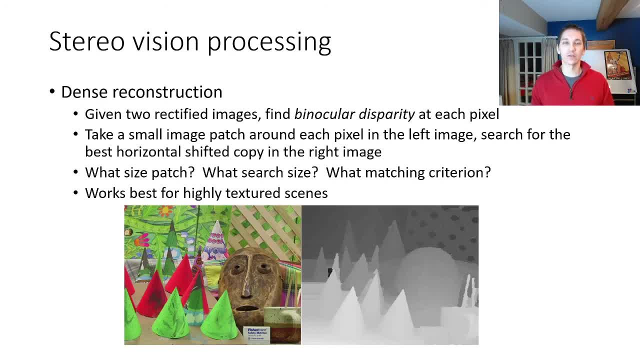 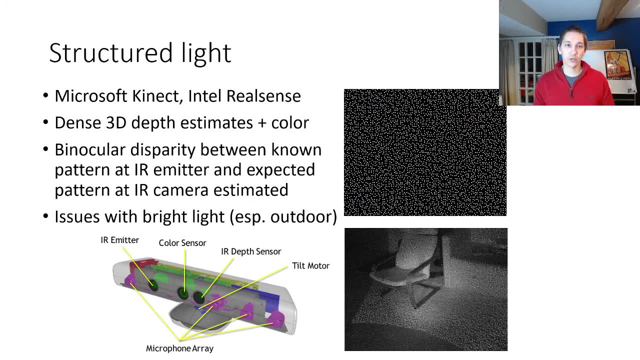 Now, if you see a highly textured scene like this, there's a lot of good matches, and so you get fairly good reconstructions. Another type of technique that is operating on a similar principle is called structured light. This became very popular with Microsoft Connect and now, more recently, the Intel RealSense line of cameras. Here they 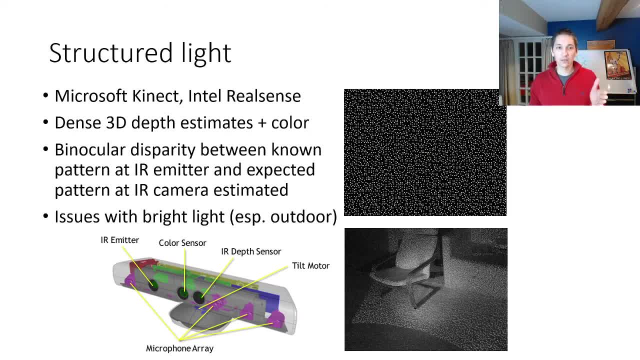 provide dense 3D depth estimates and color. They have a color sensor as well as an IR infrared depth sensor and an infrared emitter. So the emitter generates synthetic texture on the scene which allows the binocular disparity to be estimated more accurately. Now there's a baseline between the IR emitter and the 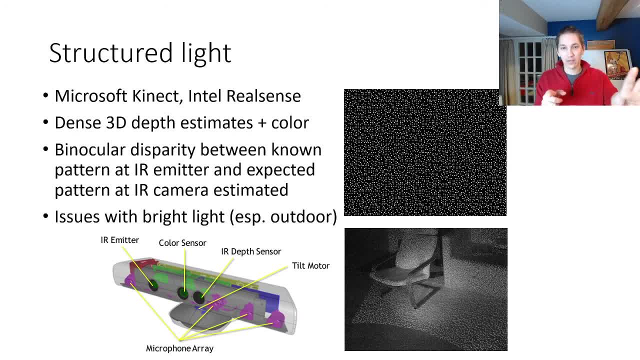 IR depth sensor. The depth sensor knows what was emitted. There's some pattern that gets emitted onto the scene, such as the one shown here, and by doing a binocular reconstruction- a dense reconstruction- you can get fairly good estimates of depth for scenes that are not too washed out. Now, if there's 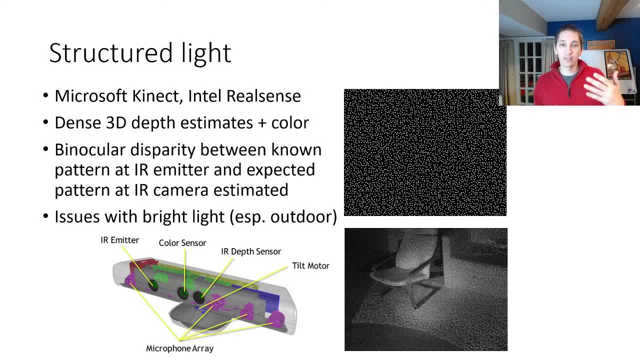 bright light, then the readings that you get back are going to be dominated by the bright light rather than the pattern that's emitted by this IR emitter, and so you end up getting poor performance outdoors. Now, if you have a set of depths and you have a set of depths and you have a set of depths and you have a set of. 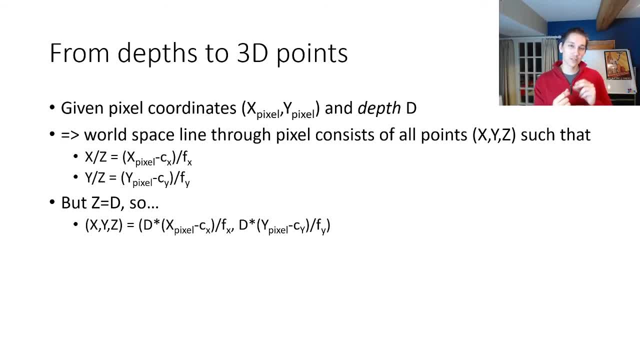 Now, if you have a set of depths and you have a set of depths and you have a set of so depth here is actually going to be not exactly the distance from the camera, but rather the distance in the forward direction only of the camera. With this 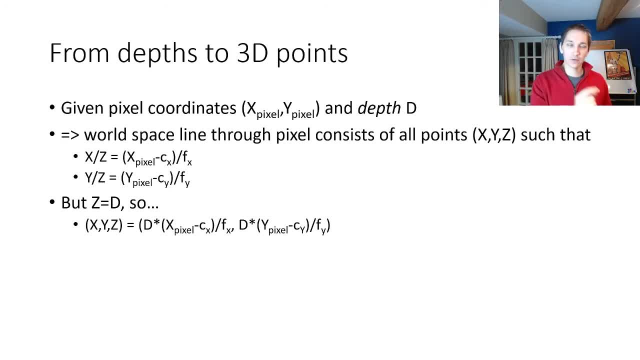 with this measurement we can figure out from a pixel coordinate and the depth at that pixel coordinate, we can figure out the world space line through that pixel. but we know the depth, we know the Z value given from the sensor and so we can just reconstruct the X, Y and Z from that point through the, through this. 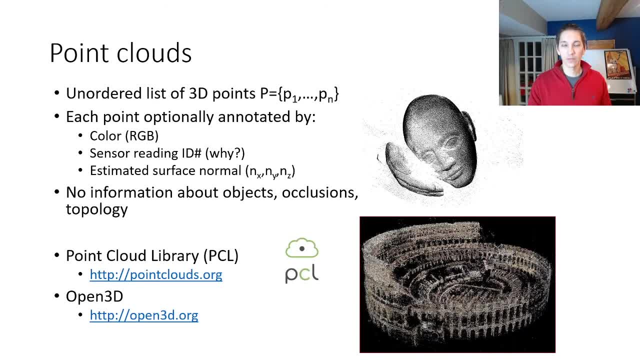 following transform. Now, with this we get what's known as a point cloud. So a point cloud is a. basically it's a list of points in 3D space. Each point can have color, some sort of sensor reading ID and surface- normal. As we've said before, these don't. 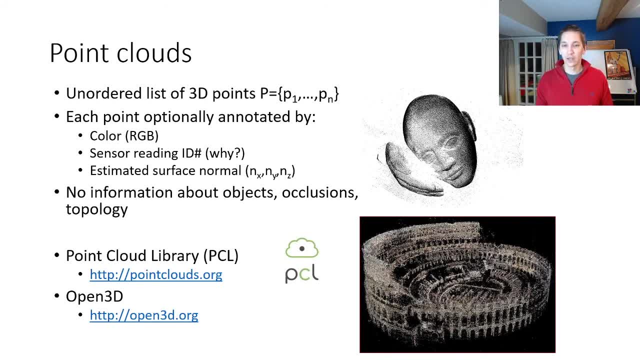 have information about which objects are in the scene, the inclusions or the topology, but in any case, these are very rich representations which are very useful for doing manipulation planning, especially A couple of characteristics about point clouds that we have to worry about. So the 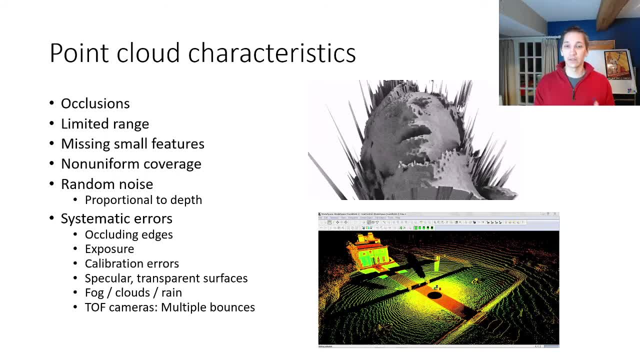 biggest one is occlusions. We oftentimes don't see a lot of. you know, there's a lot of missing data, especially these sorts of shadows. So we basically see the front sides of objects. we don't see the backs. we don't see what's behind. 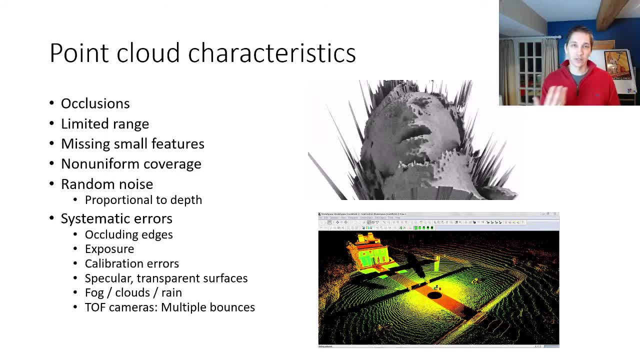 them. There's also oftentimes limited range, depending on the type of sensor that you have. They'll also miss small features due to the resolution. So if we're trying to pick up a very small object, they may be sub pixel size in the of the image and in that case we'll likely miss them. They also have non-uniform coverage of the. 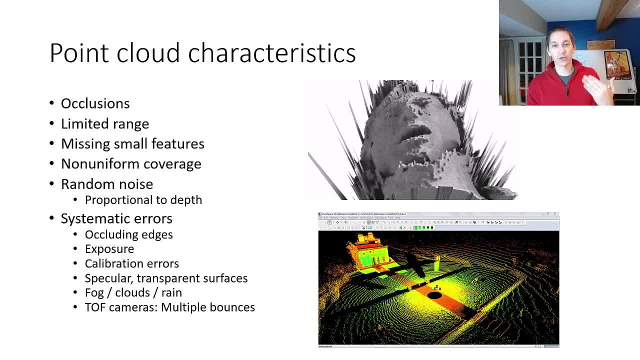 3D scene, so objects that are farther away will have a sparser sampling in terms of pixel of points per unit area, compared to objects that are close to the sensor, And there's also going to be a lot of noise in these images and they're typically proportional to depth, and so you'll 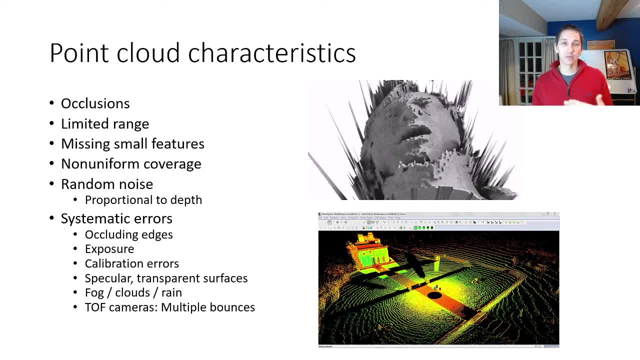 oftentimes see characteristics like one percent depth measurement error or two percent depth measurement error, meaning that you know if you are at one meter away, then you're expecting to see, for example, one centimeter of error in the depth. There's also systematic errors, including 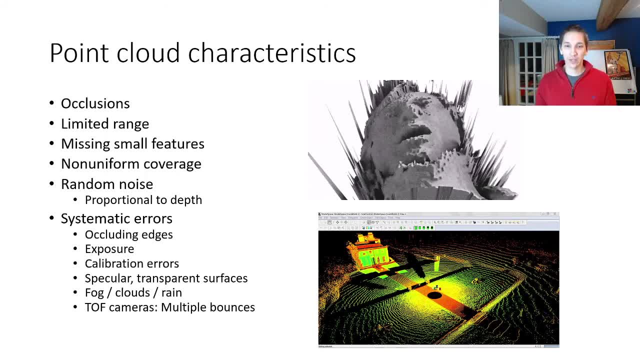 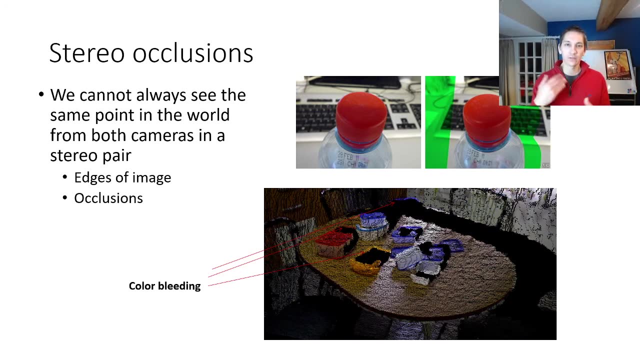 these occlusions, exposure, various calibration errors and reflective surfaces. so oftentimes you'll get, you know, bogus readings or no readings from these types of sensors, these disturbance. So we have to be a bit wary of how to do with these types of systematic errors in our data. So one very important one is stereo occlusions. 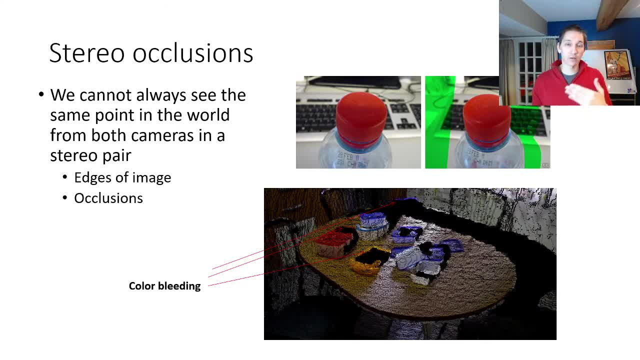 because many times these point clouds are generated through stereo reconstruction. Again, because of stereo disparity, the points that you can see in one camera image are not going to be exactly the same as the points you can see in the other camera image. So 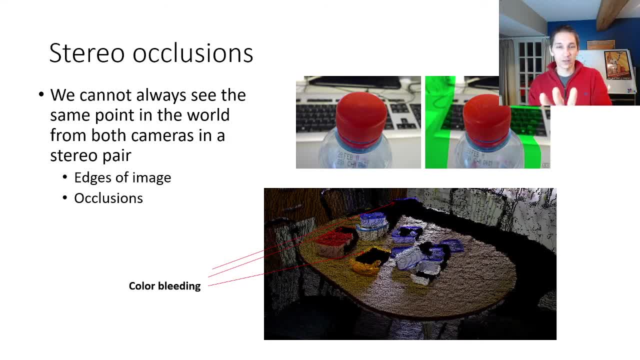 if we look at these two images of this water bottle and this keyboard, in the back there's parts of the keyboard that are not seen in the left image. There's also parts of the like both behind the bottle as well as those on the extreme side of the image. So